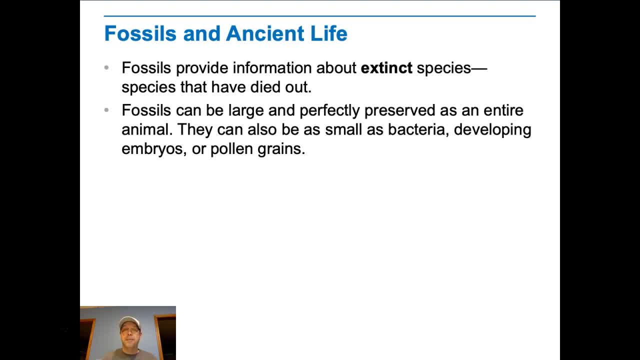 perfectly preserved, like an entire animal, like the woolly mammoth that was discovered over in Russia in the permafrost. They can be small, like bacteria, little embryos, little pollen grains. Sometimes fossils are just pieces of an organism, not a whole organism: Teeth, parts of the body. 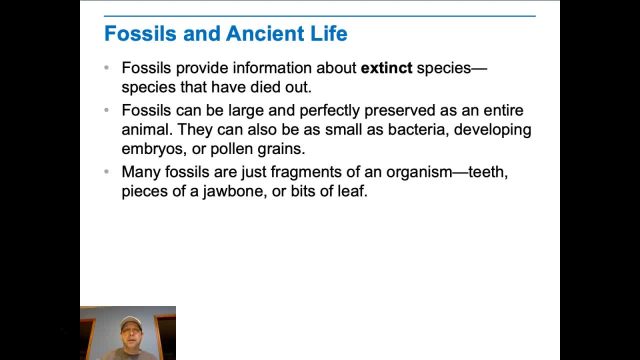 bone, a piece of a leaf, an imprint of a part of a leaf. Sometimes we just see the trace, things that may be an organism left: Footprints, burrows, tracks or even droppings that have become fossilized. So most fossils are preserved in what we call sedimentary rock. Some are preserved in 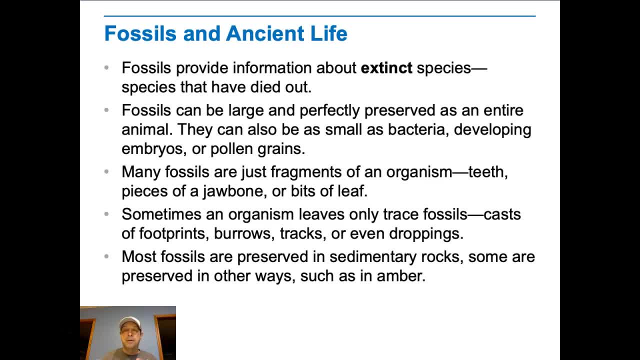 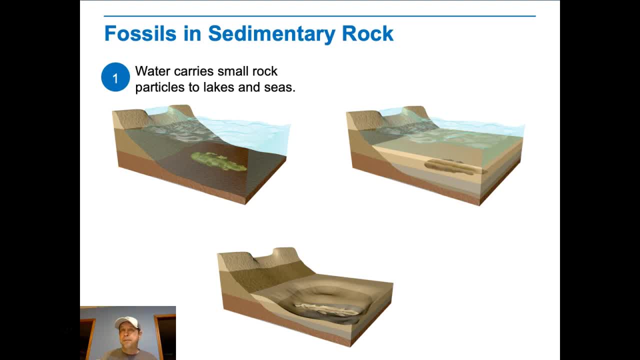 other ways, like in amber, which is fossilized sap, and other places like the frozen in the permafrost or things like that. So fossils form in sedimentary rock. So water carries small rock particles into a lake or into a shallow sea. Dead organisms are buried by layers. 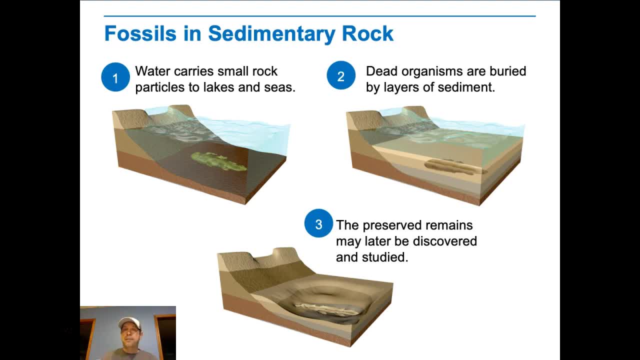 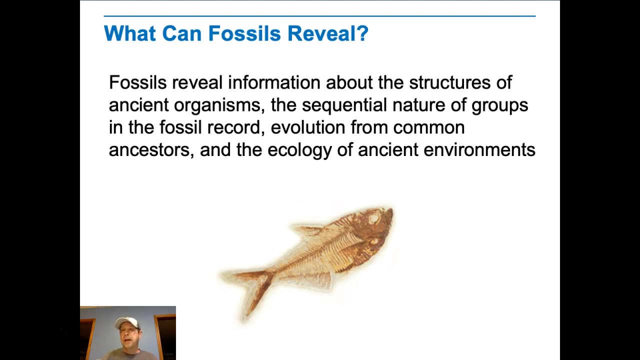 of sediment. The water and stuff compress the sediments and they eventually convert the layers of sediment into rock, which then preserves the fossils within them. So what can fossils tell us? What do they tell us about things? They can tell us what they look like. 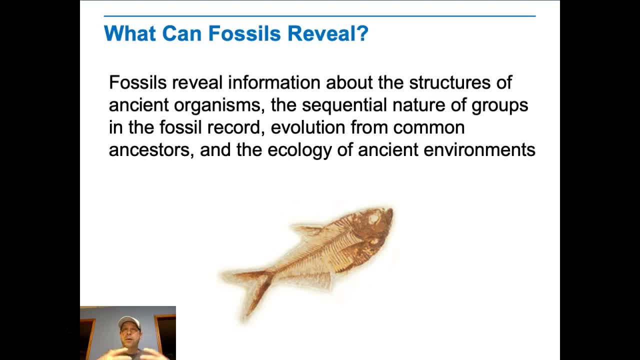 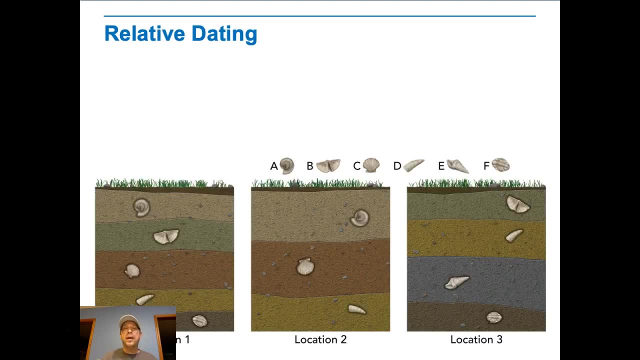 They can tell us the sequence by which they evolved from a common ancestor. They can tell us about their environment, where they lived, how they lived, things like that. So when we go to figure out how old a fossil is, there's two kinds of dating. we use Relative dating and 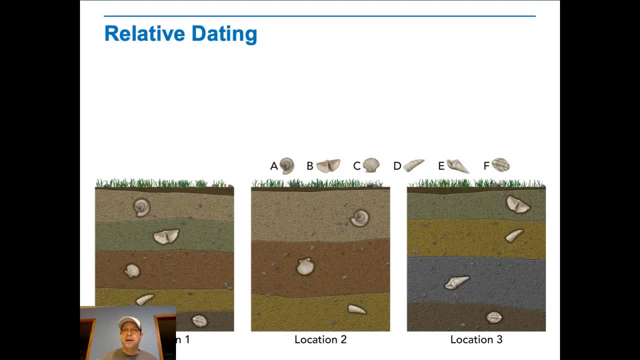 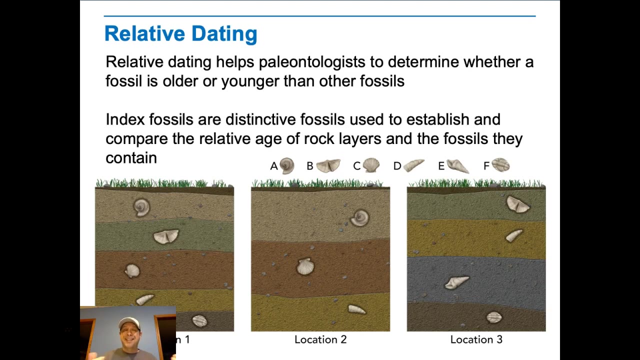 radiometric dating or using radioactive elements. So relative dating basically involves determining whether a fossil is either older or younger than other fossils in the same area, So it relies on what we call index fossils, Fossils that are found pretty much all around the 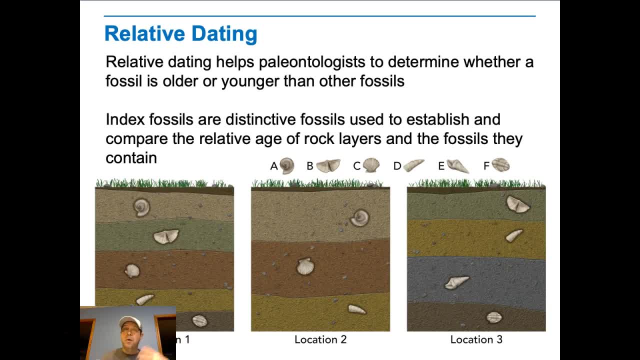 area in the layers, And so we know how old these fossils are approximately, and that can help us determine whether the layers are in the correct order or whether there's been some type of geological process that's shifted them. But they can help us again figure these things out. 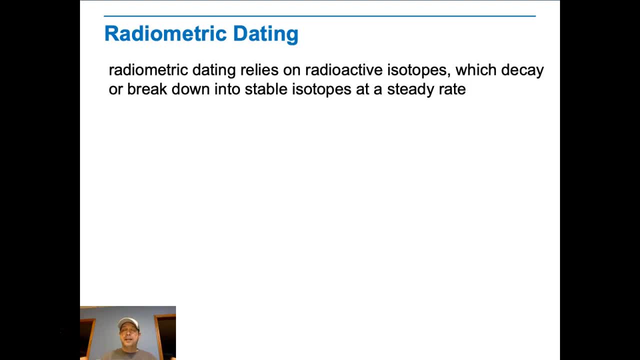 Radiometric dating gives us a more precise date. It relies on the fact that radioactive isotopes break down in a predictable and a steady way from a radioactive isotope into a stable isotope. Now the difference is in radioactive isotopes. they give off energy in the form of neutrons or protons. excuse me, 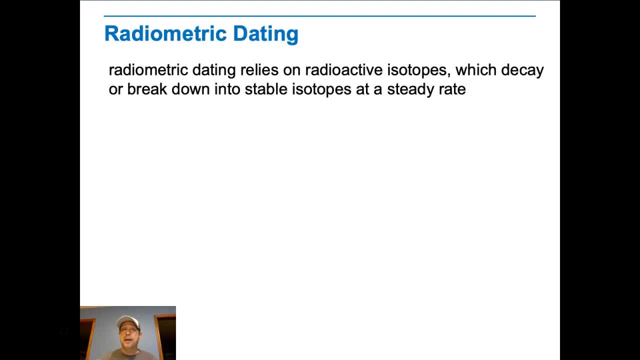 And as they do that, it changes the atom from one type to another. So the rate at which they break down is called the half-life. It's the time it takes for half of the radioactive atoms in a sample to decay from the radioactive form to the stable form. 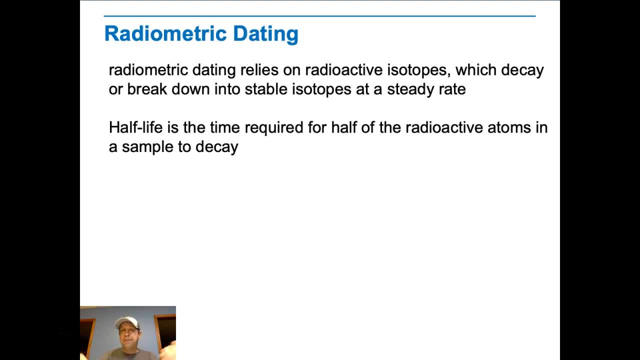 So let's say the half-life is 20 years. Half of it after twenty years is going to be converted into the stable form In another twenty years. half of that half and so on and so on. And so we can look at the ratio of the stable to the radioactive isotopes to determine how old a sample might be. 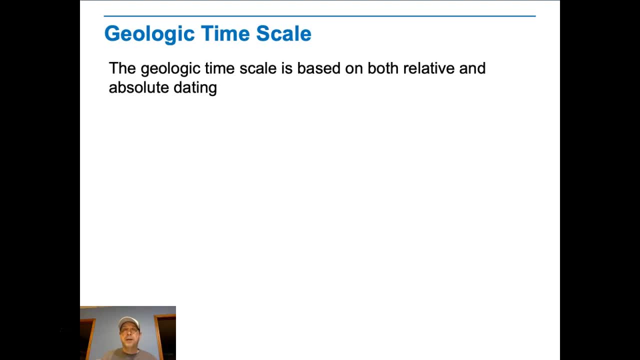 So there's something called the geological times scale, which is based on both relative and absolute dating data, And the geological times scale is just going to be a data variable of the time scale. there are major divisions called Aeons, Eras and Pyramids. 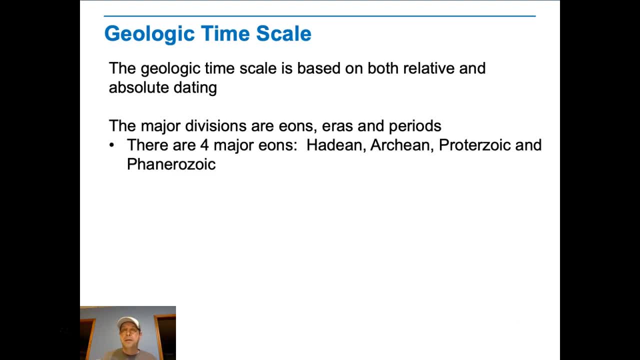 There are four major Aeons: the Hadron, Archeon, Proteozoic and Panherozoic. Hadron is when rock first formed, Archeon, life first appeared, Proteozoic, stable continents began to form and Eukaryotes evolved. 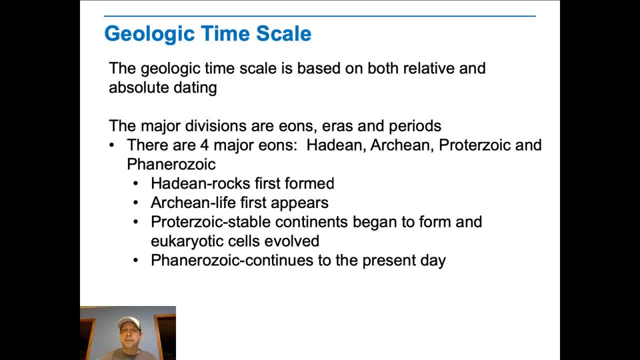 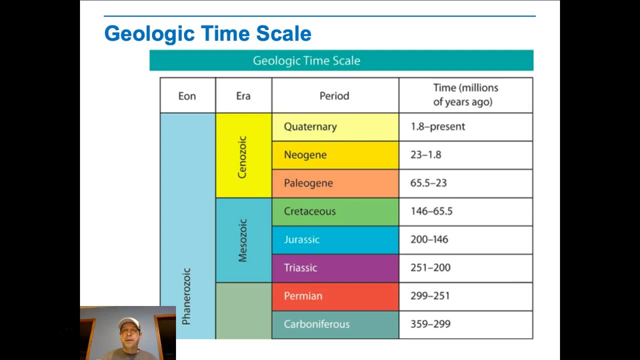 And finally, the last one is from the end of the Proteozoic until present day. Aeons are divided into eras and eras are divided into periods. So here you can see on the graphic the breakdown here. So at the top we're looking at present day. 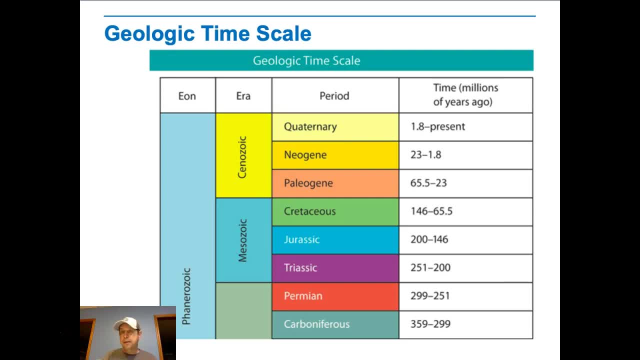 So the present day era is the Cenozoic Quaternary Period. You can see how it breaks down. It breaks down into the Mesozoic and so on. You've got: the Mesozoic is when the dinosaurs roamed, Cenozoic is when mammals first evolved, and so on and so forth. 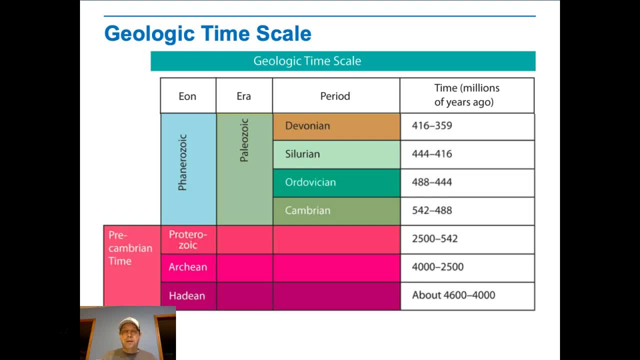 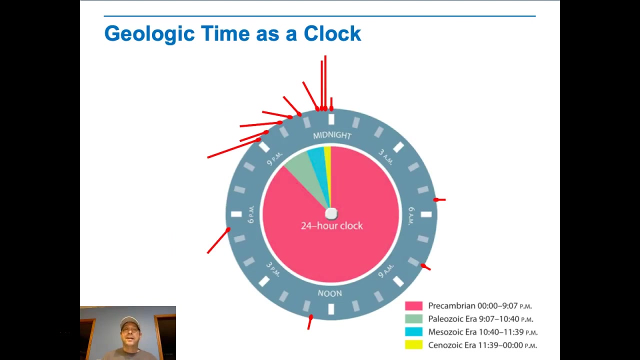 Here we can see the Paleozoic Era, And then the Precambrian Time is also broken down as well. So three of the four Aeons are what we call Precambrian Time. So one thing that's useful is to kind of think of the history of Earth. 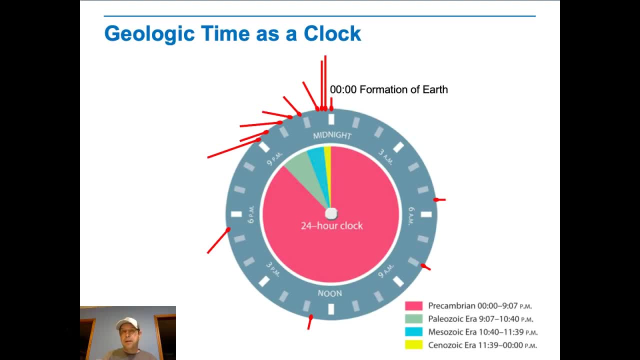 as a 24-hour day. So Earth forms at midnight, at 530 in the morning, the first living cells. We have evidence of those. You can see again on the clock. you can see the breakdown with the chart here with the different eras and so on. 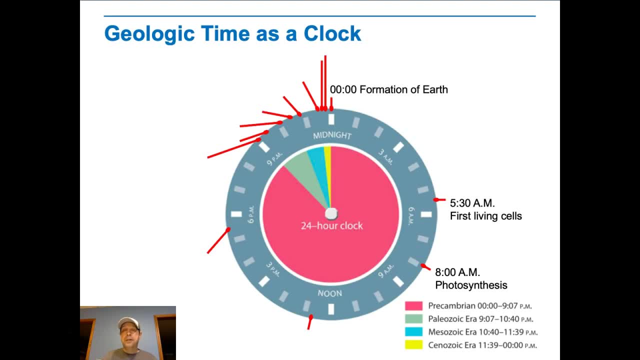 Eight o'clock in the morning, photosynthesis evolves and we start getting oxygen in the atmosphere, And about 1248 in the afternoon eukaryotes show up. Multicellular organisms show up, about 530 in the evening, Chordates, which are things that have a notochord, which is us. 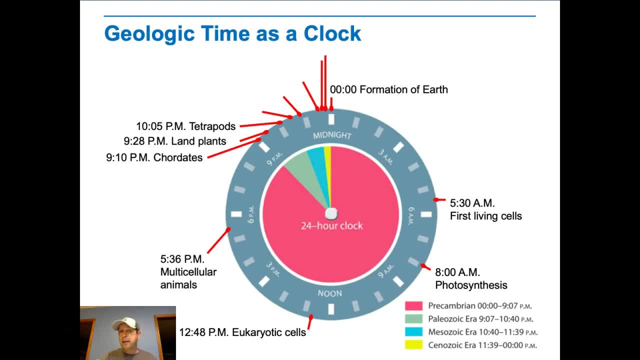 Land plants, pteropods, land animals, Dinosaurs show up about 1045.. Mammals: about 1058.. So they haven't been around very long at all. Flowering plants: 1120.. Dinosaurs go extinct at 1139. 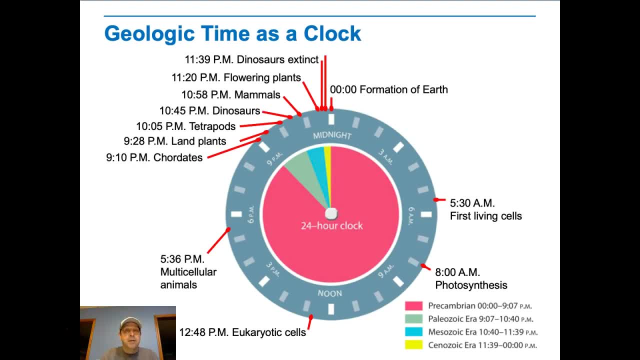 We think they went extinct a long, long time ago, But on the scale it's pretty recent. And finally, 1158 and 56 seconds is when we show up. So one of the things we know from studying geology is that 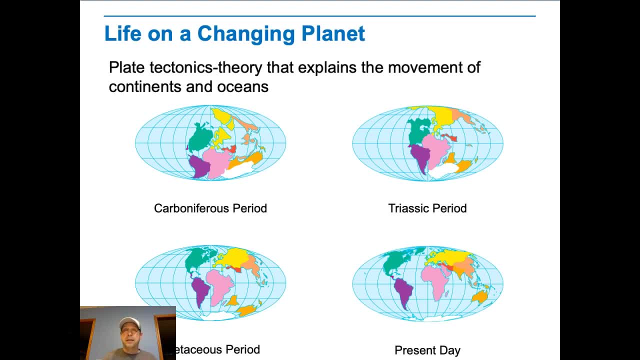 the land masses of the continents are not set in place. There's something called plate tectonics, which is a theory that explains the movement of the continents and how that affects the oceans. We start with Pangea and it spreads apart until current day. 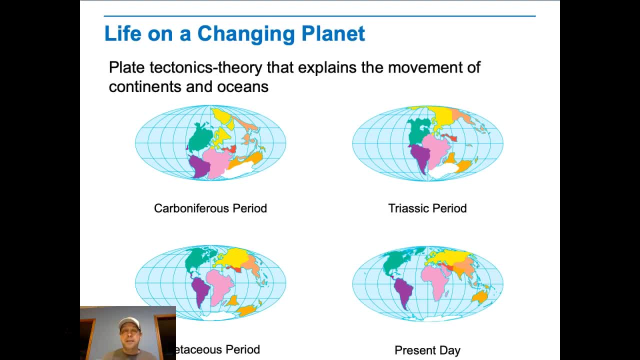 And again that changes the environments on the land masses as they separate and they become more internal or more on the coast, They shift in their latitude and longitude, And all of those things affect the climate, which affects the kinds of living things that lived in different parts of the world.